shipment will move from one particular source to one particular destination. It may be from S1 to D2 or S1 to D3 or S2 to D3, or from S2 to D3 or S2 to D3, or from S2 to D3, or from S1 to D3, or from S2 to D3, or from S2 to D3 to S1 to D3. 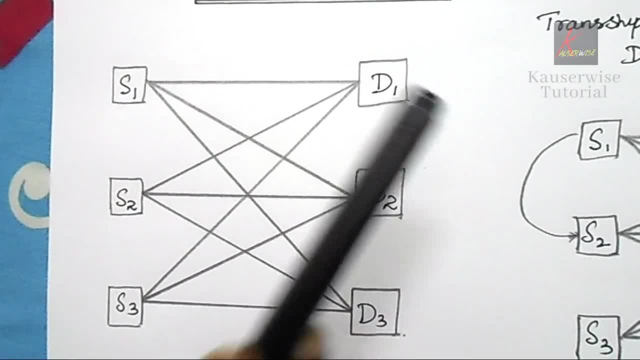 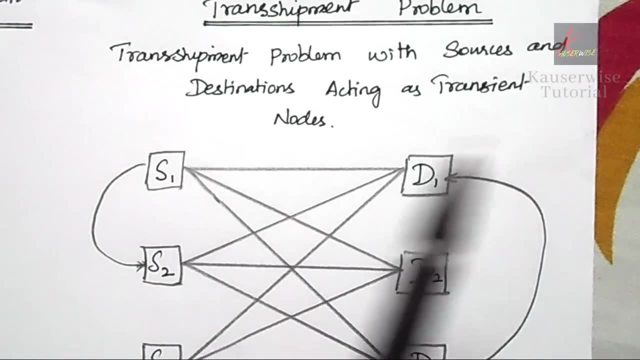 The shipment will directly move from one particular place to one particular destination. So this is the model for transportation. Now look at the model for transhipment. problem with sources and destinations acting as transient node. See, in this method the shipment will 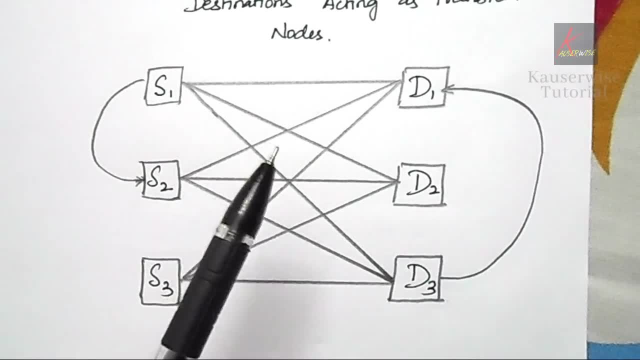 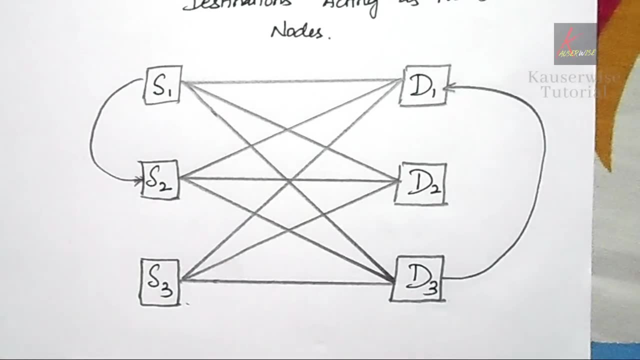 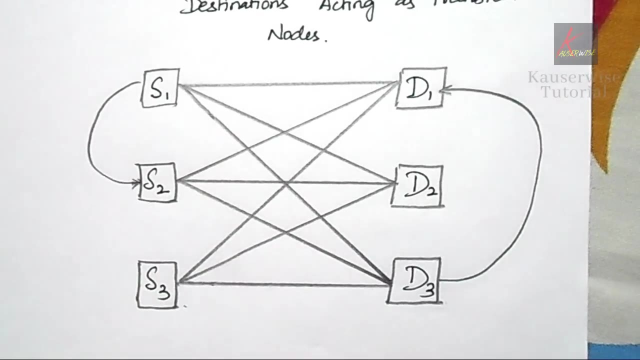 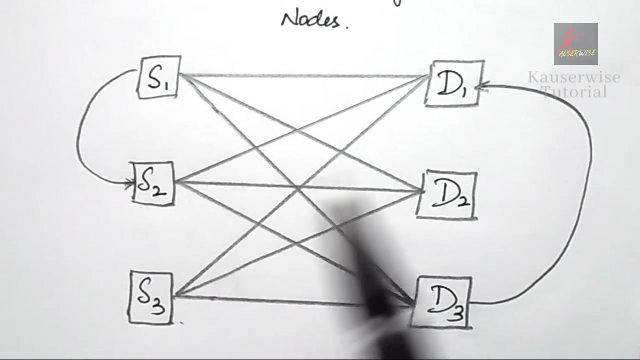 pass through one or more intermediary nodes before it reaches its desired destinations, which means so this method allows the shipment passes through from one particular place to sources, to another source and from one destination to another destination before it reaches to the desired destination. so the intermediary nodes can be sources and destinations themselves. okay. 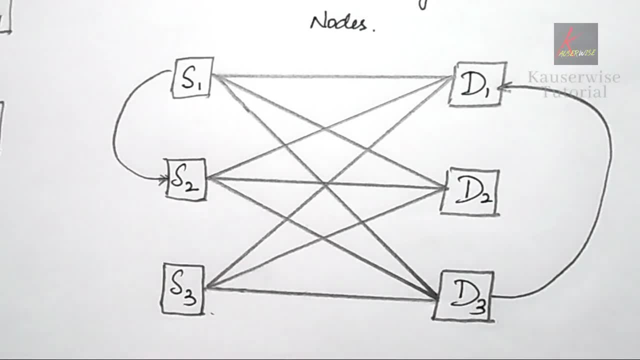 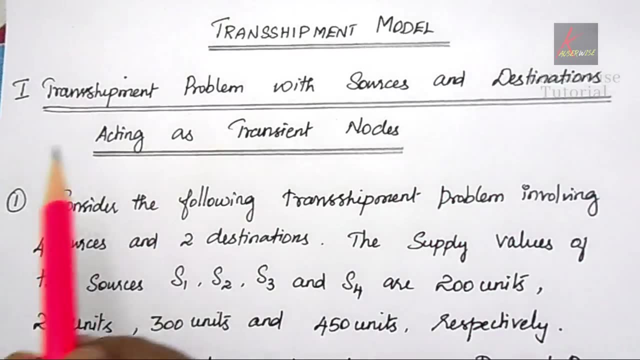 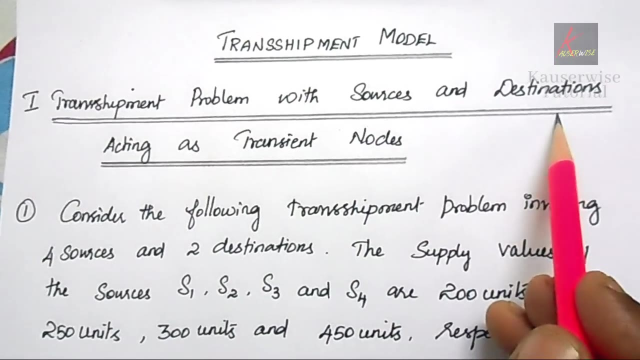 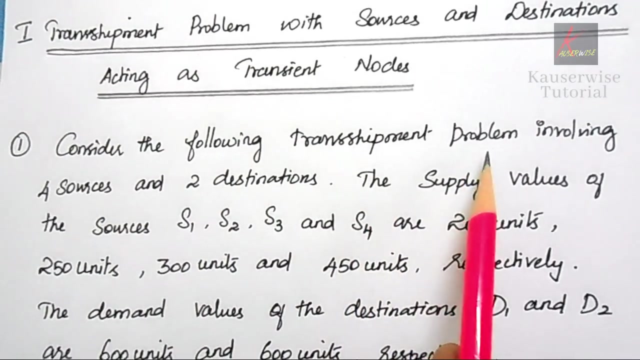 now let us see the problem for better understanding. see the problem for the first method: transhipment problem with sources and destinations acting as transient node. so transient node means intermediary node here, sources and destinations acting as a intermediary node. look at the problem. consider the following: transhipment problem involving four sources and two destinations. 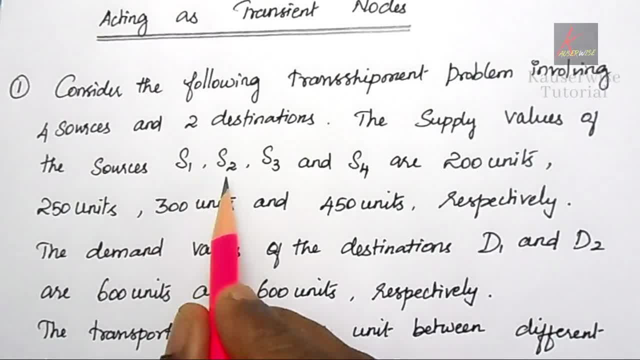 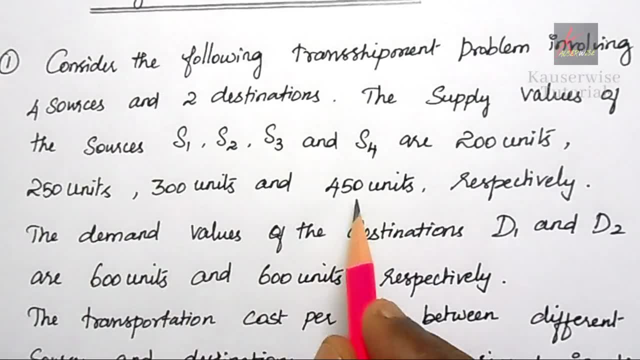 the supply value of the sources s1, s2, s3 and s4 are 200 units, 250 units, 300 units and 450 units. so these are the supply values for four different sources and destinations acting as a intermediary node here. sources and destinations acting as a. 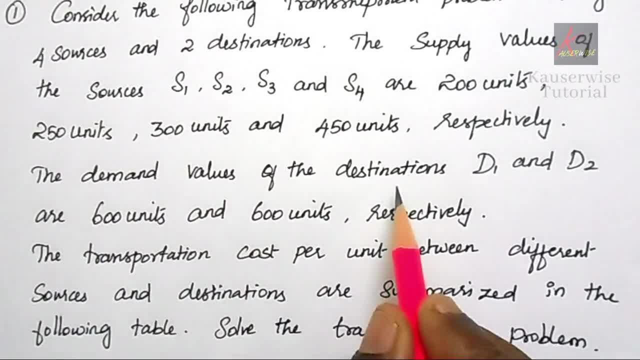 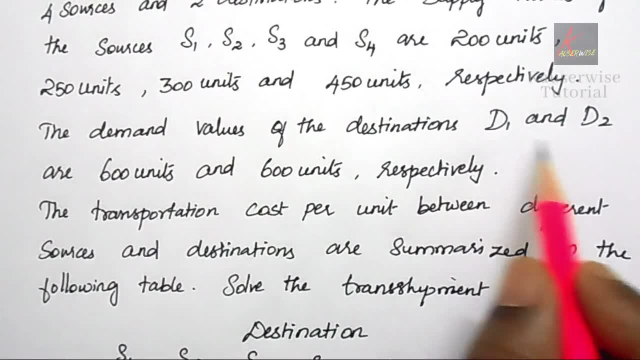 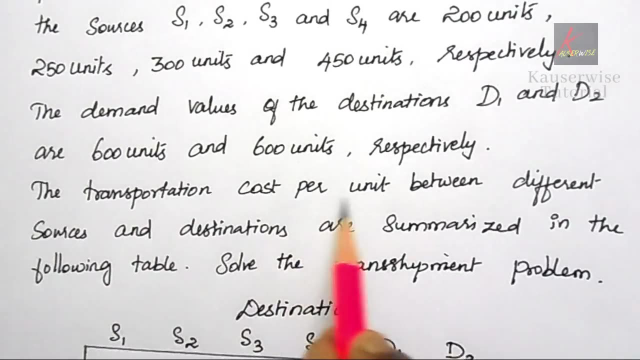 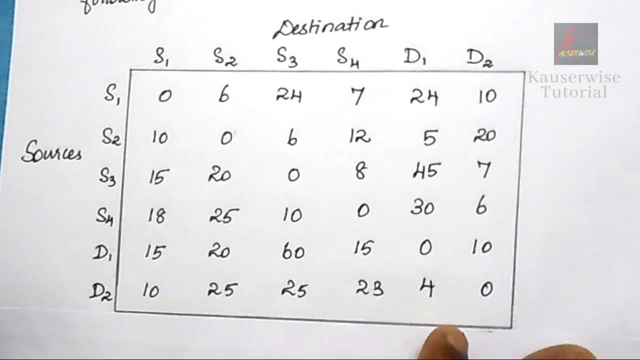 and then the demand values of the destinations d1 and d2 are 600 units and 600 units respectively. so demand for destination 1 and 2 is 600 and 600 respectively. the transportation cost per unit between different sources and destinations are summarized in the following table: see the table. 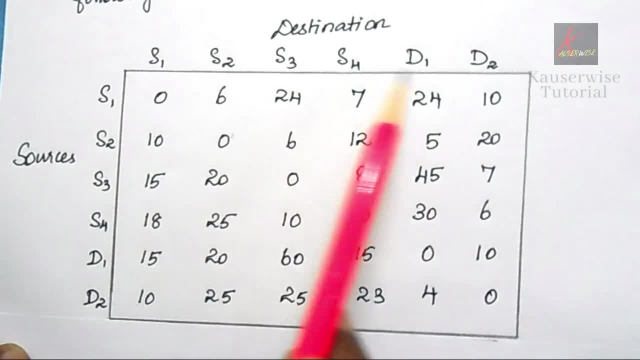 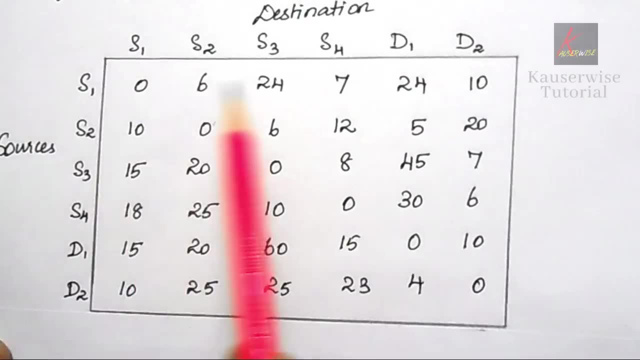 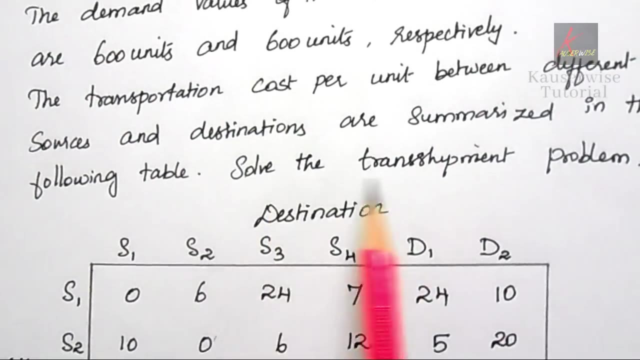 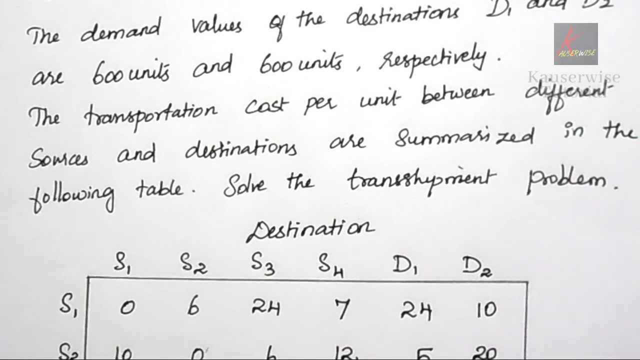 which is given in the problem. here, there are four sources and two destinations. okay, so these are the various transportation cost per unit between different sources and different destinations. okay, now, with this information, they ask you to solve the transshipment problem. okay, now we are going to solve the transshipment problem by using simple steps. now let us see. 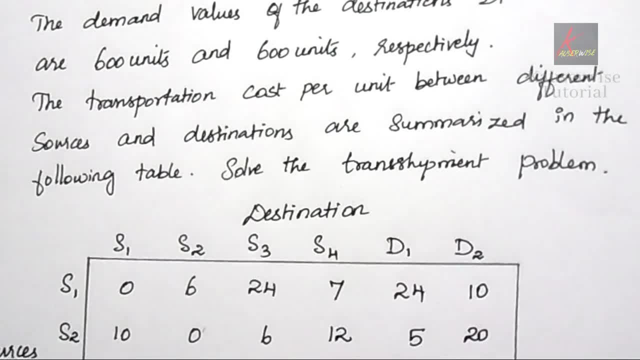 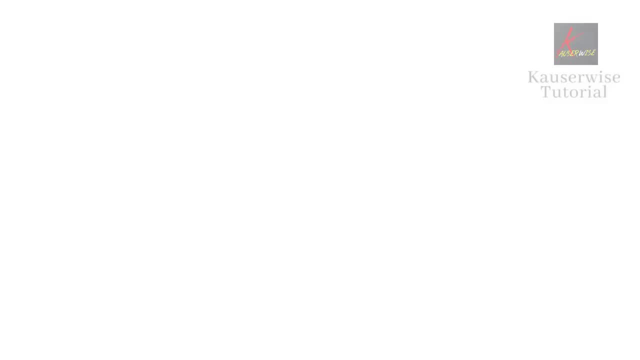 the steps which is required to solve the transshipment problem. see, there are four steps are there to solve this method. we will see one by one, along the line of the transshipment problem. so let us see the first step. the first step is to check whether it is balanced or 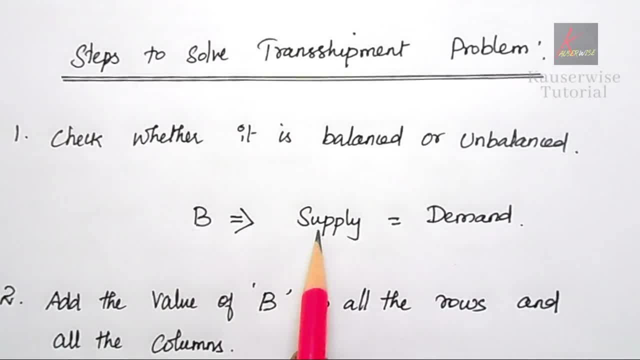 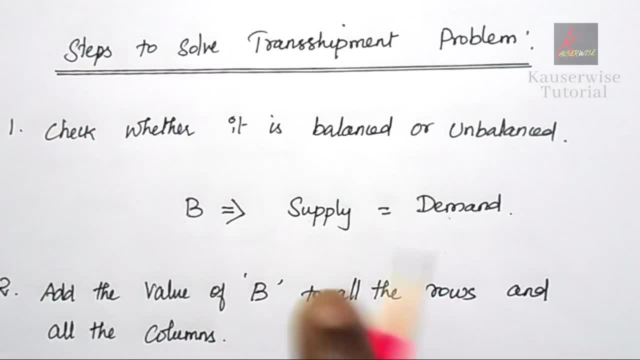 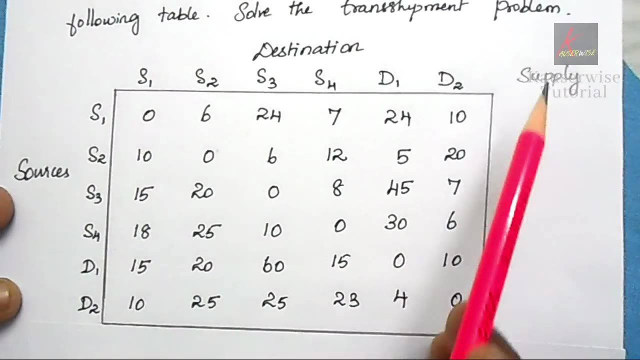 unbalanced. balanced means supply value is equal to demand value. the sum of total supply is equal to sum of total demand. now let us check whether the problem is balanced or unbalanced. the first step is you have to check whether the supply is equal to demand. okay, look at the problem. 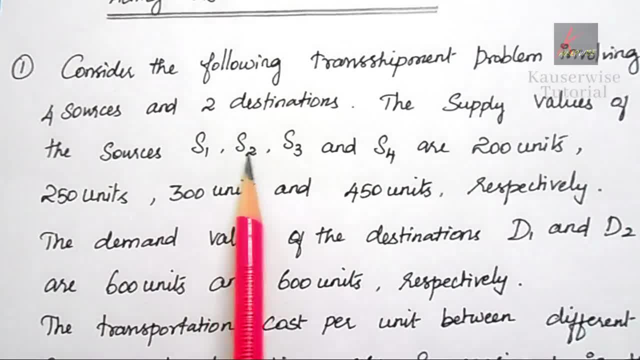 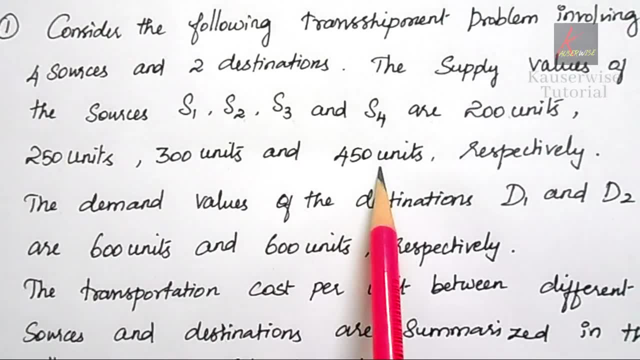 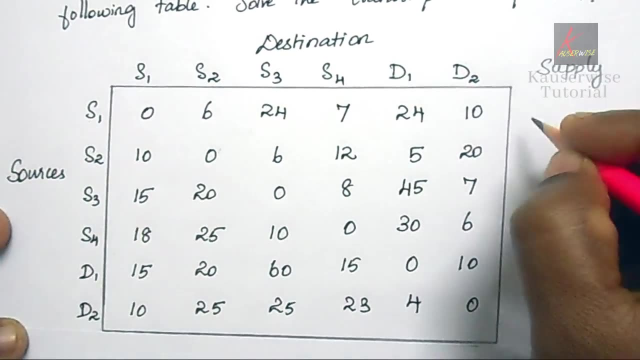 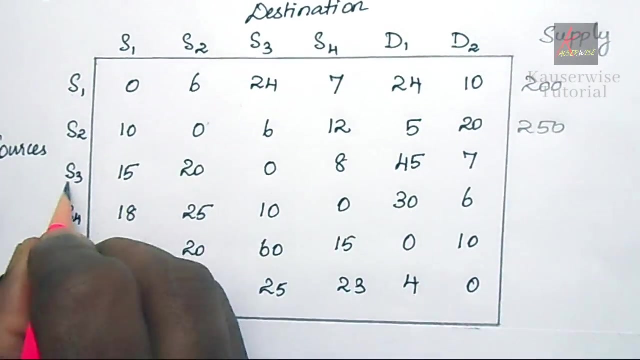 see the supply value of the sources. s1, s2, s3, s4s are 200 units, 250 units, 300 units and 450 units. so in this table you have to write the supply values for sources one. what is the supply? 200 units, okay. for s2, 250 units. for s3: 300 units. for s4: 450 units. so this value is equal to demand value. 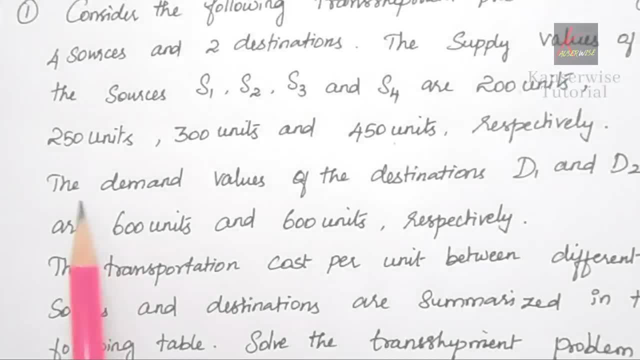 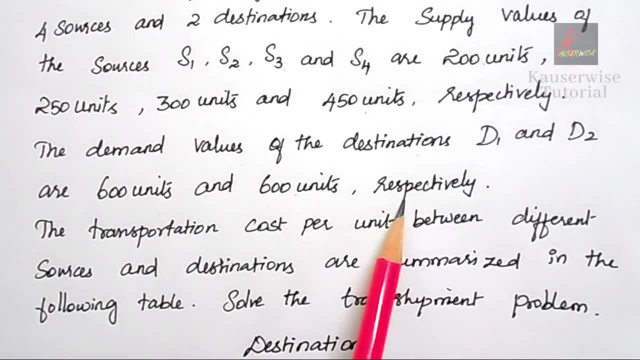 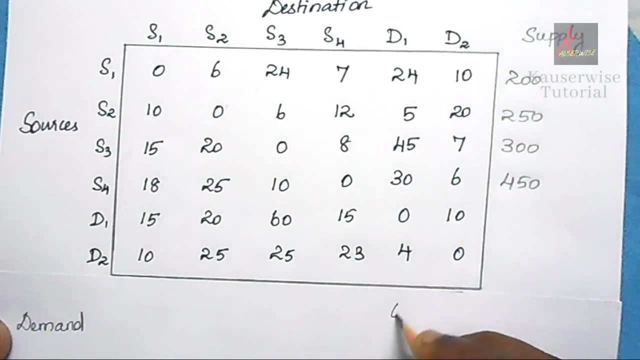 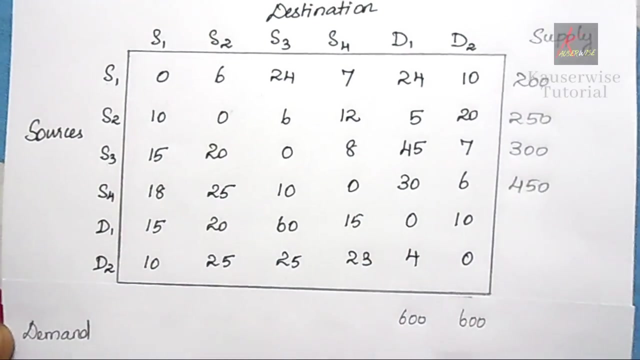 this information is given in the problem. now see the problem. the demand value of the destination d1 and d2 are 600 units and 600 units respectively. see here the demand for destination 1: 2 is given: for d1: 600 units. for d2, also same 600 units. okay, after entering the value for supply and demand. 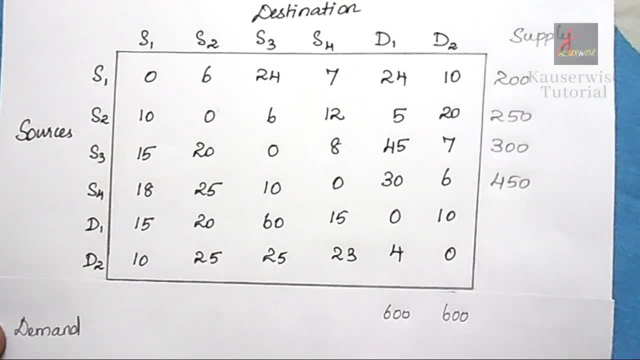 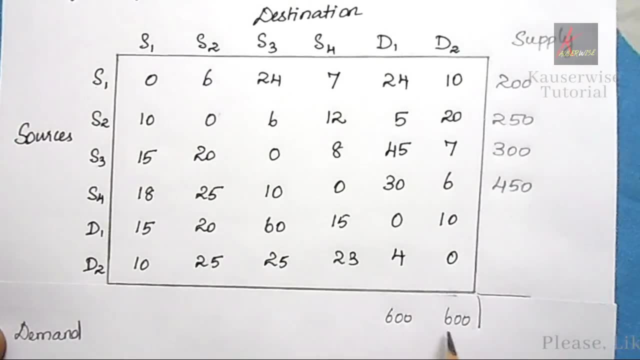 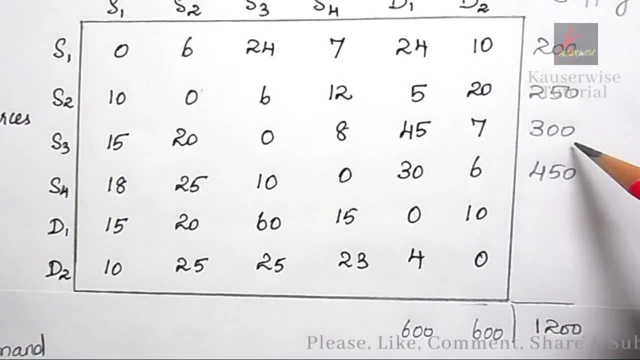 now you can check whether it is balanced or unbalanced. balanced means both demand and supply will be equal. now check the demand: is 600 plus 600 1200. okay. now check the supply: 200 plus 250 plus 300 plus 450, you'll get 1200. so this problem is balanced to one. 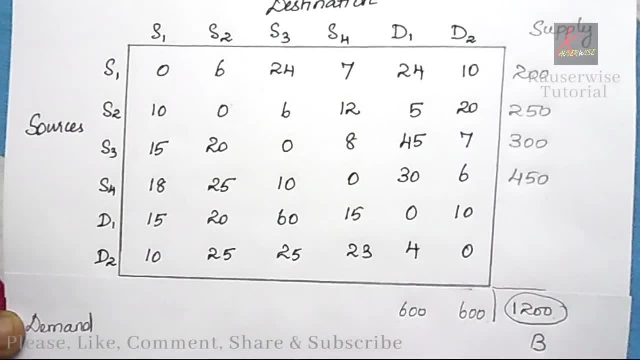 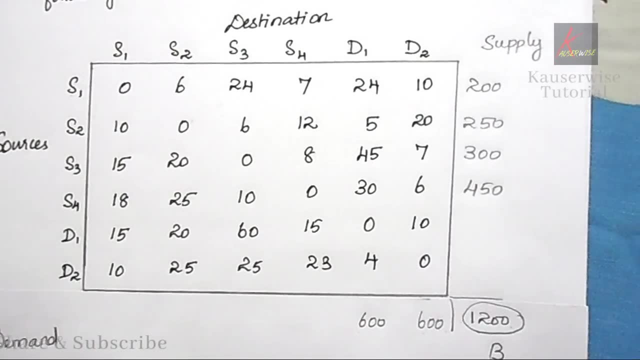 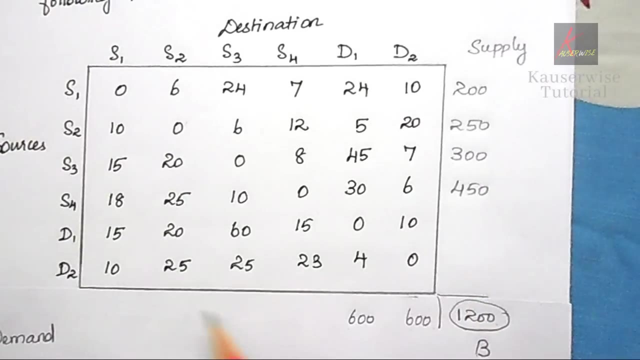 so consider this value as b. since it is a balanced problem, this will be considered as b. see, if the problem is unbalanced means unbalanced means supply will not equal to demand. in that case you need to add either dummy row or dummy column with zero values. 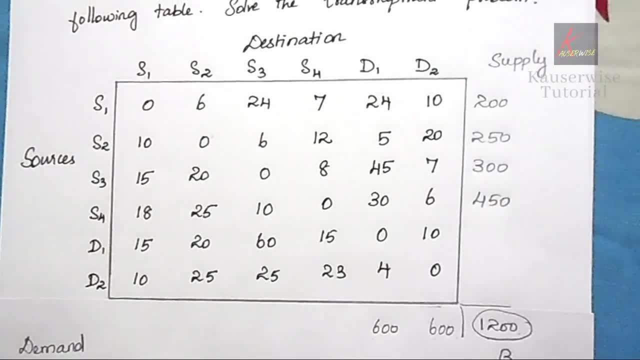 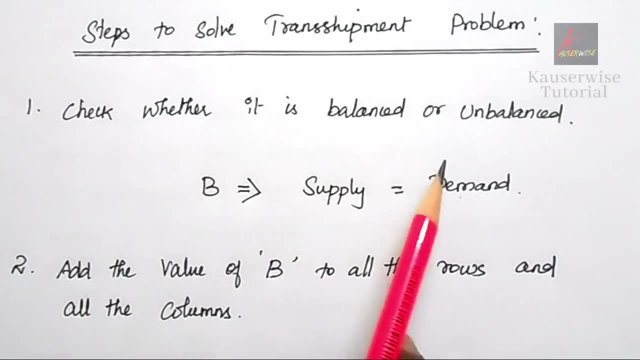 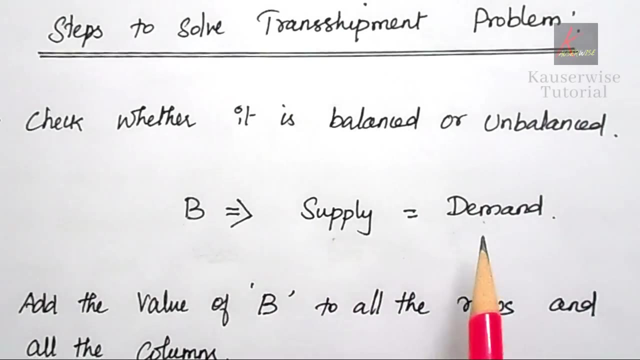 in order to convert unbalanced into balanced one. that problem we'll see separately in another video. look at the step, the first step we have completed, that is, we have verified whether it is balanced or unbalanced. so our problem is balanced one. here. the total value of supply and demand is 1200. 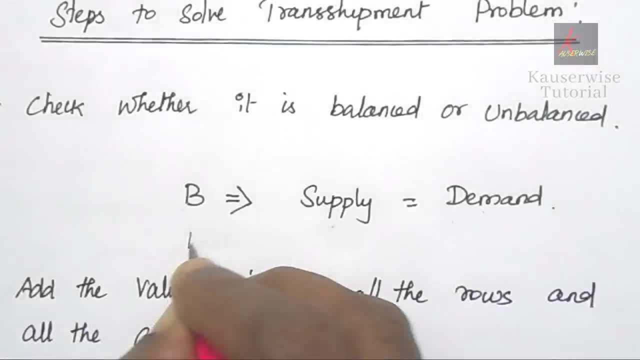 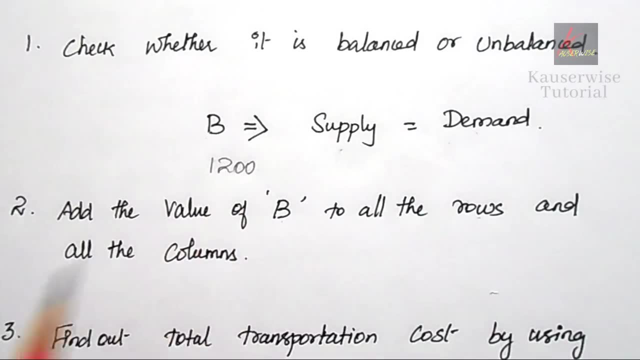 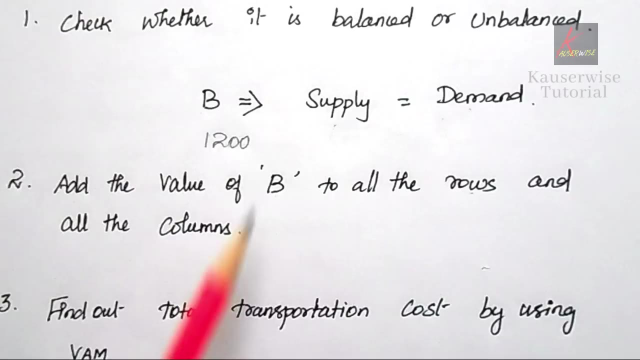 so the b value will be 1200. okay, now look at the second step. after we find out the b, that is 1200- now we need to add the value of b to all the rows and all the columns. now let us see how to do this. look at the problem now. we need: 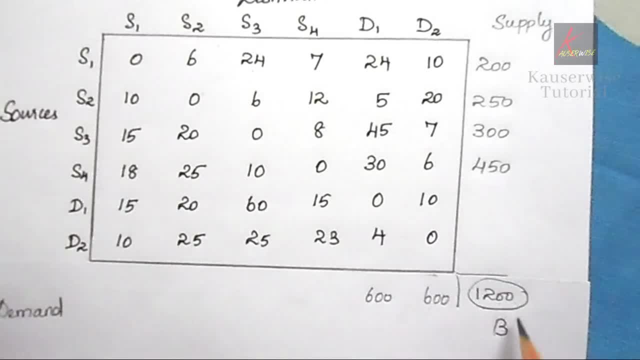 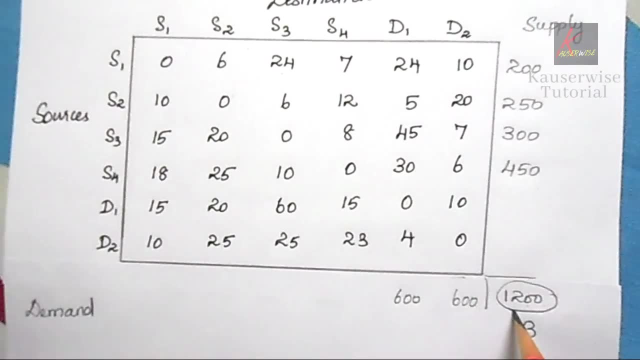 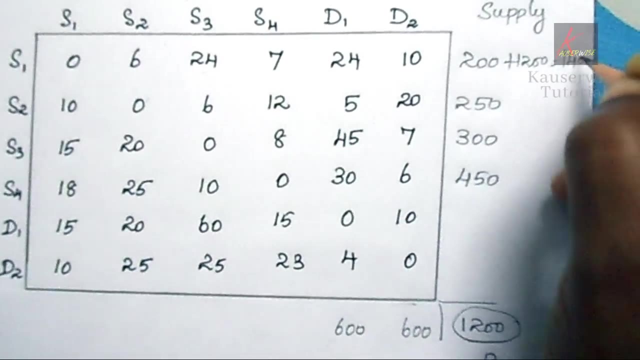 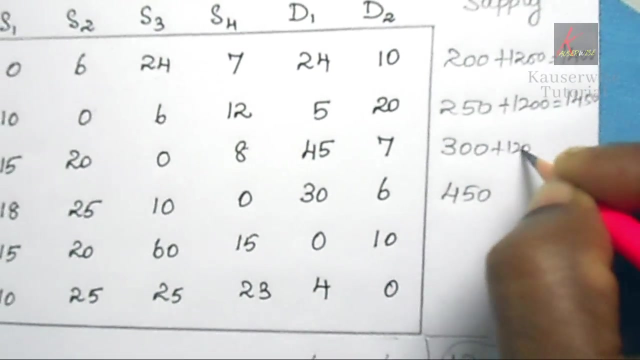 to add this value, that is, total demand and supply value. this need to be added in all the row values and in all the column values. now i'm going to add 1200 in all the rows. okay, for the first step. first row plus 1200, you'll get 1400. in the next row, 1200 is equal to 1450. again here, 1200 is equal. 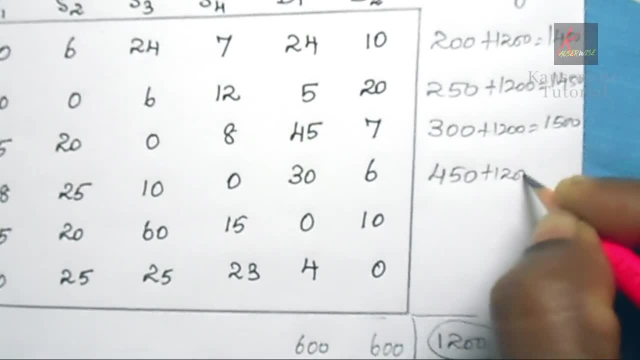 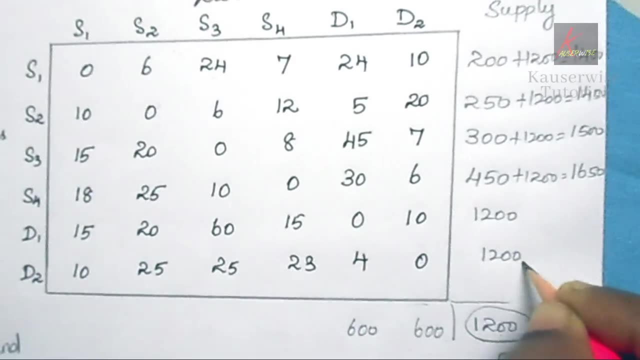 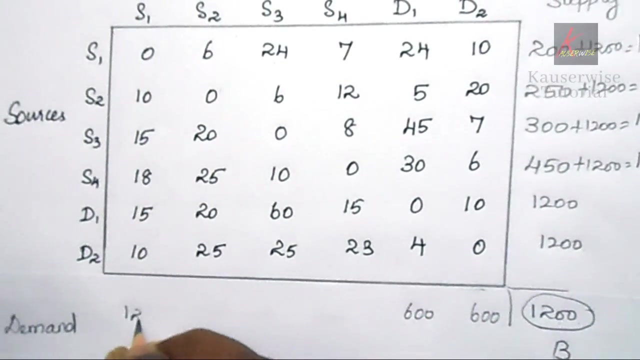 to 1500 plus 1200 is equal to 1650. here nothing is there now. simply, you can add 1200- 1200. in the same way, we need to add this value for the all column values for the first column, 1200. 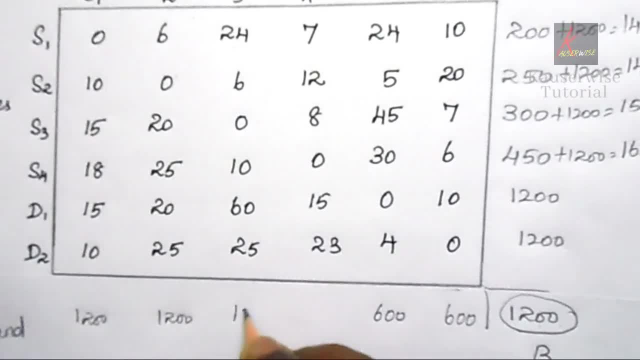 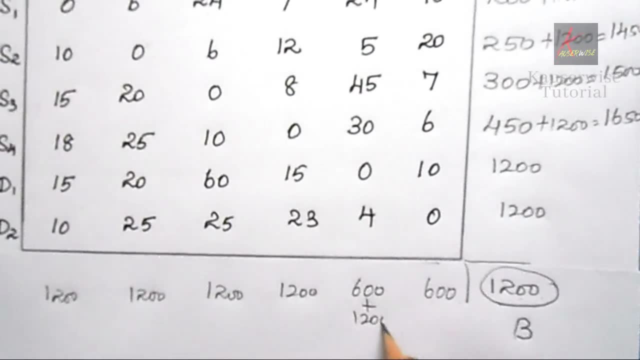 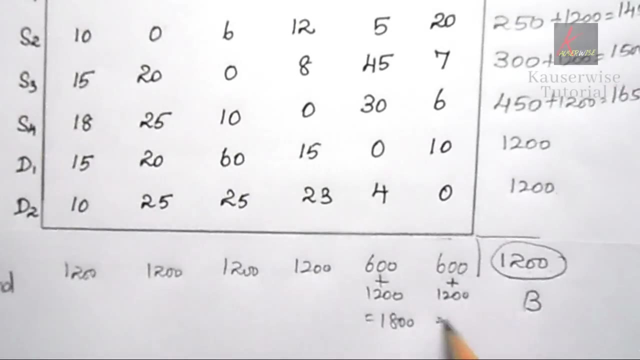 for the second column: also 1200, 1200, 1200. for the fourth column: already 600 is there now plus 1200, you'll be getting 1800. for the last column: already 600 is there, plus 1200, you'll get 1800. 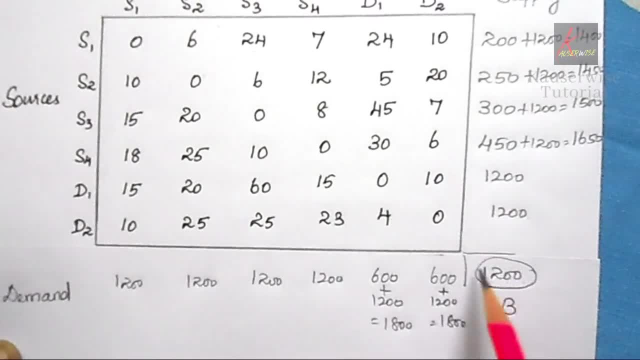 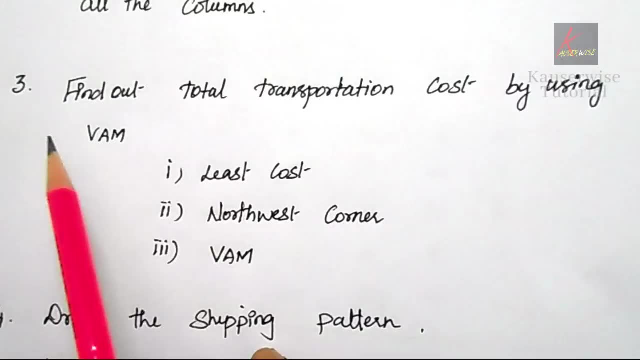 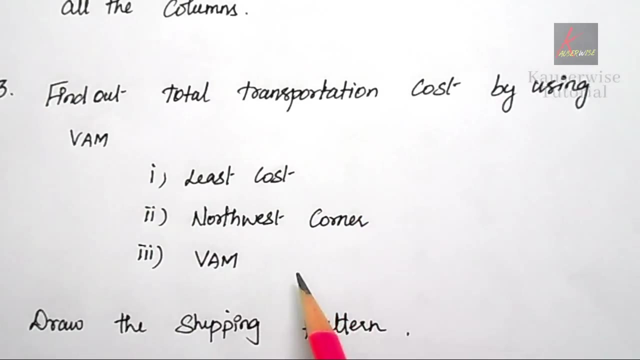 this is the second step. okay, so we have added 1200 in all the row values, as well as column values. look at the next step. the third step is to find out total transportation cost by using vam. see, there are three techniques are there to find. 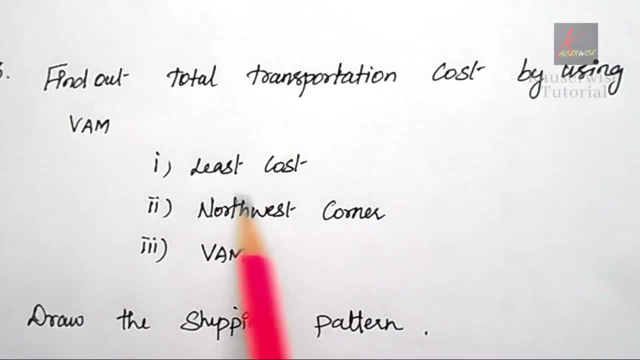 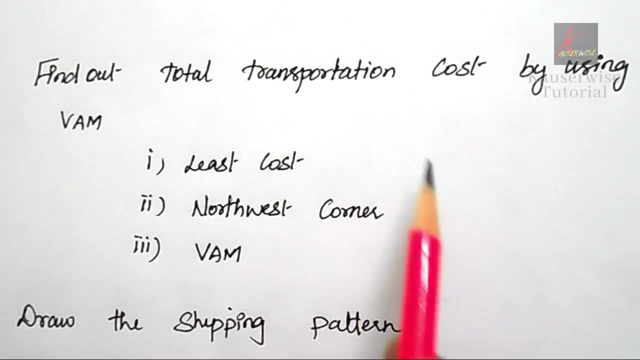 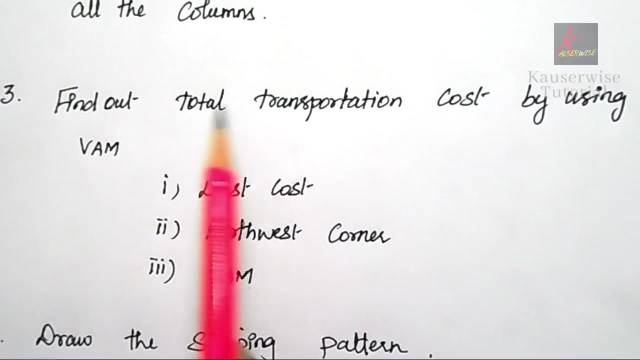 out total transportation cost. that is, the first one is least cost, second one, northwest corner. and third one is ogles approximation method. among three techniques, vam solution will be the least one. now we are going to apply this method to find out the total transportation cost. see, now i'm going to 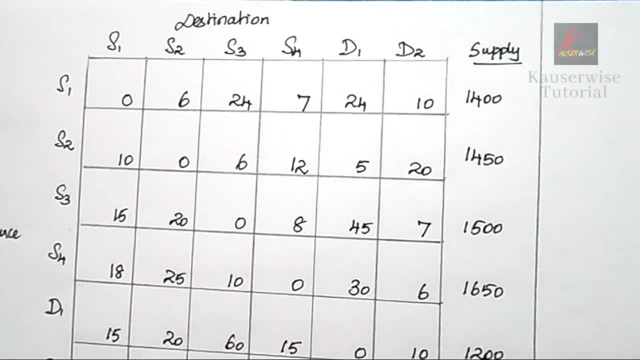 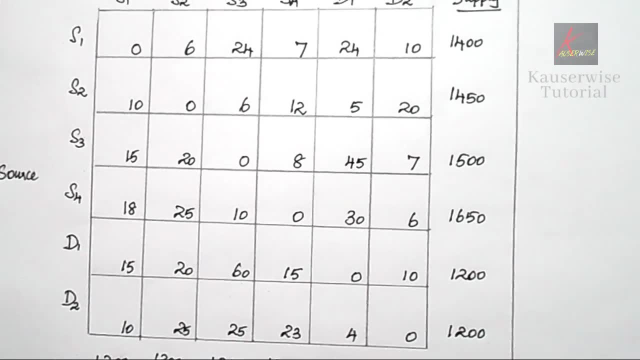 solve the problem by using vam method. see, i am going to apply this method to find out the total transportation cost. i already uploaded a separate video for transportation problem with three different techniques. okay, if you want to know about step by step procedure, kindly watch that video. it is there. 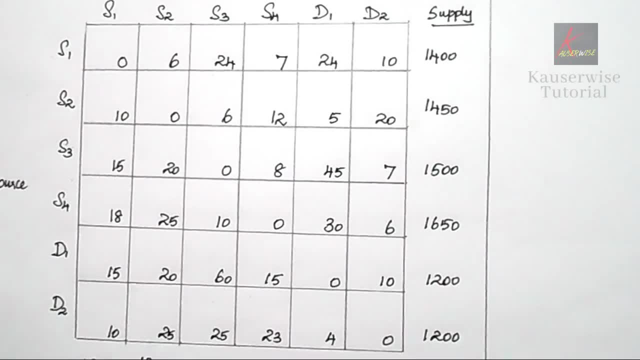 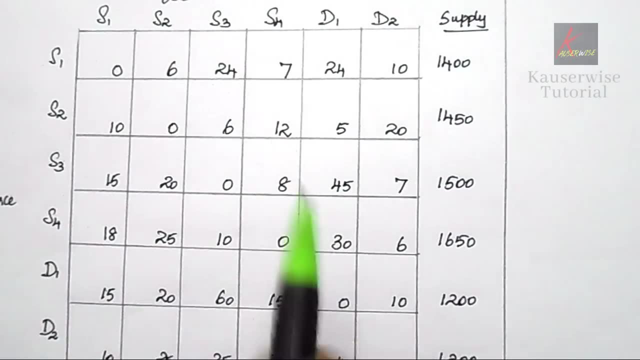 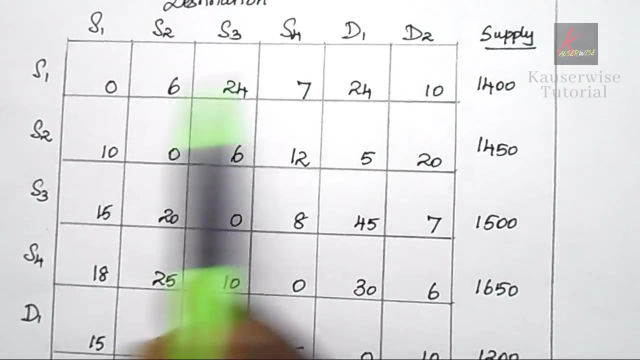 in the playlist. so now i am going to just solve the problem by using vam method. look at the matrix. first, we need to find out the row difference and column difference by comparing the least value with the next least value. look at the first row. the least value in the first row is zero. 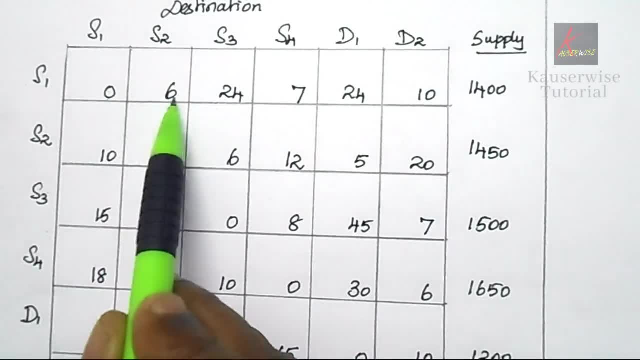 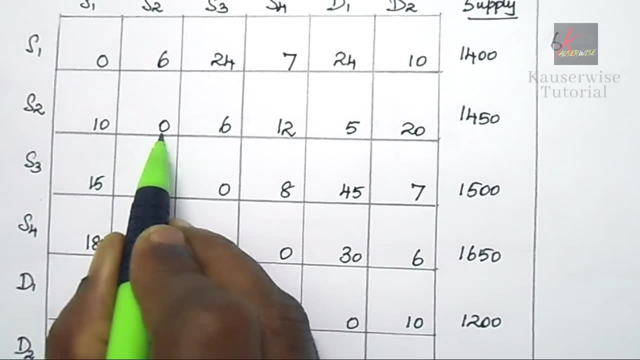 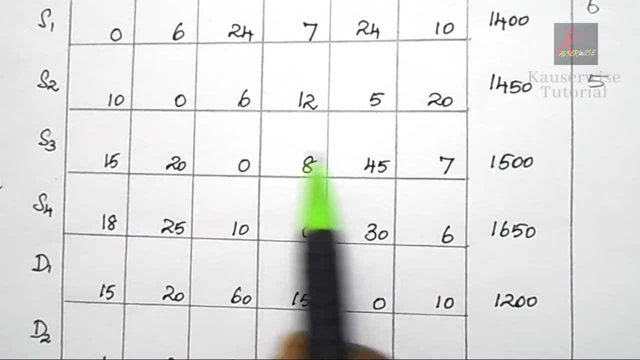 the next least value is six. now what is the difference? six. so write six here in the same way. in the second row, the least value, zero. next least value five. difference five. in the third row, the least value is zero. the next least value is seven. so difference seven. in the fourth row, the least. 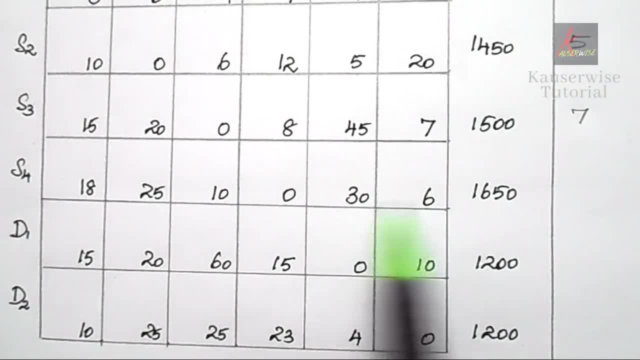 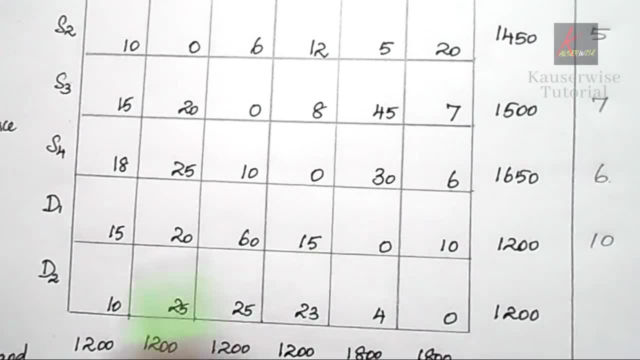 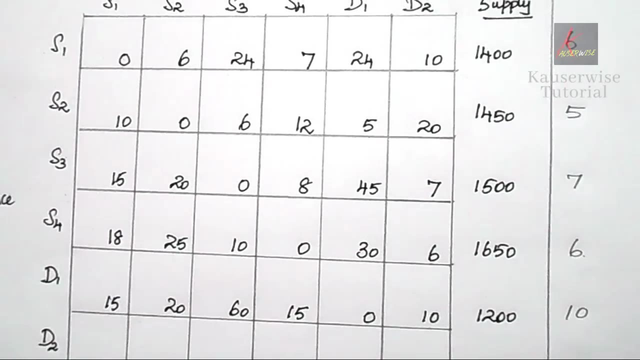 value is zero. the next least value is six. so difference six in the next row: zero and ten. difference ten in the last row: zero. four, difference four. in the same way we need to find the difference for column also. look at the first column. the least value is zero, the next: 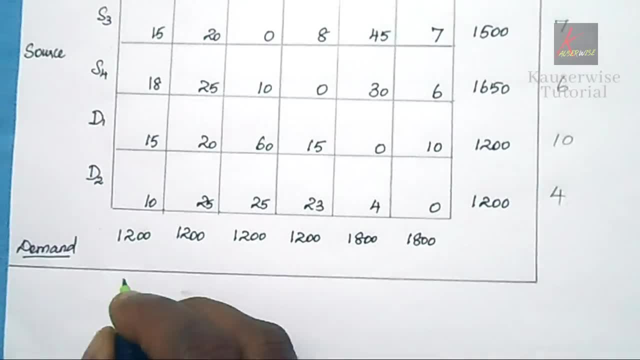 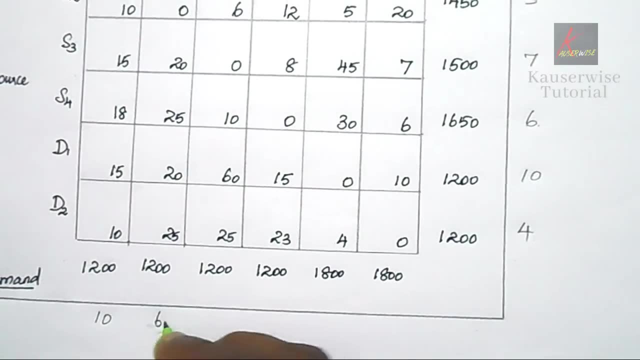 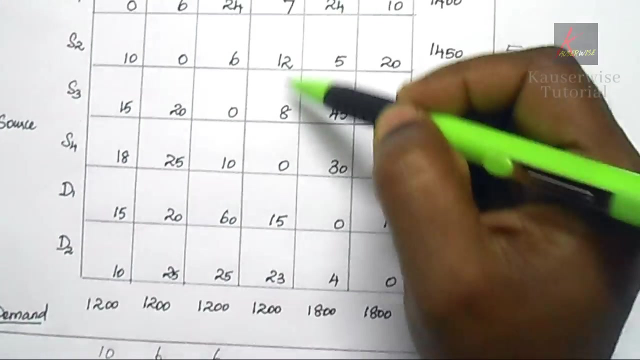 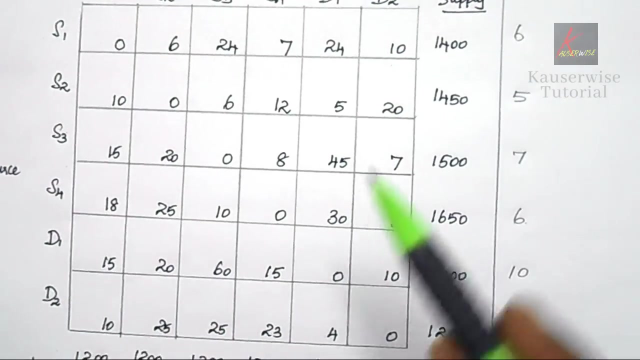 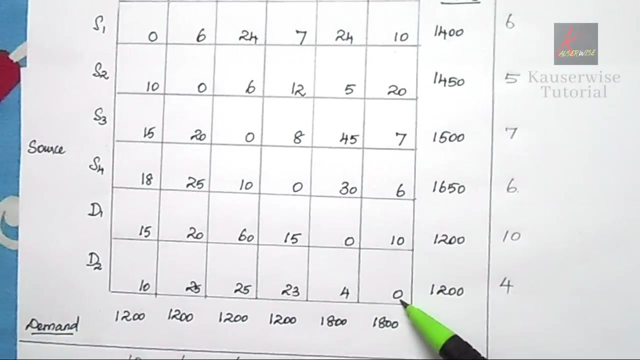 least value is ten. so difference ten. for the second column: zero, six, difference six. the next column: zero. next value six. difference six. in the fourth column: zero and seven. difference seven: see in the next column. the least value is zero, next value four, difference four. in the last column: zero and six. 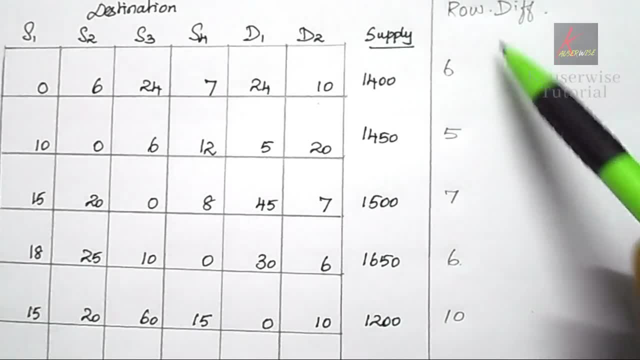 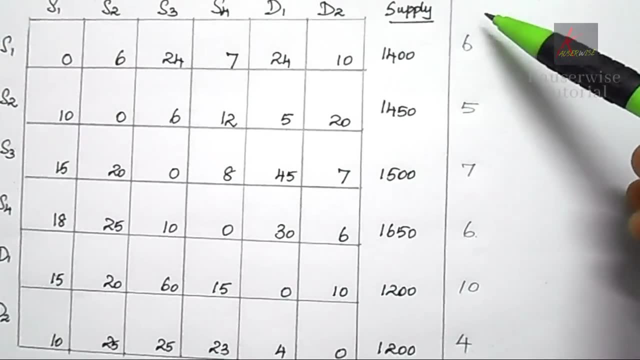 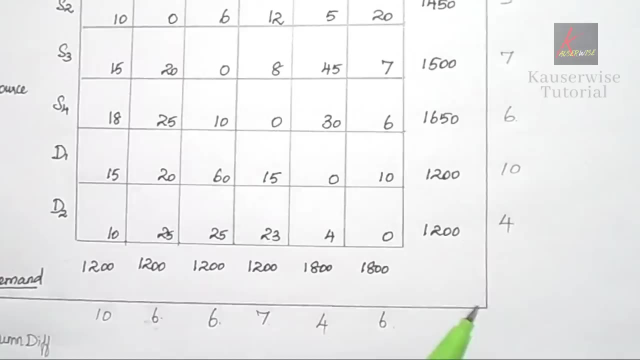 difference: six. okay, after find out the row difference and column difference, the next step is you need to select the maximum value among the difference: see the row difference. the maximum value is ten. look at the column difference: see here also, we have got ten, see. in case of time, you can select any one value randomly. so here i am going to select this. 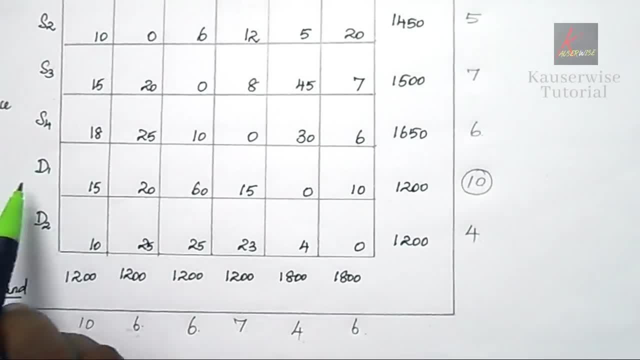 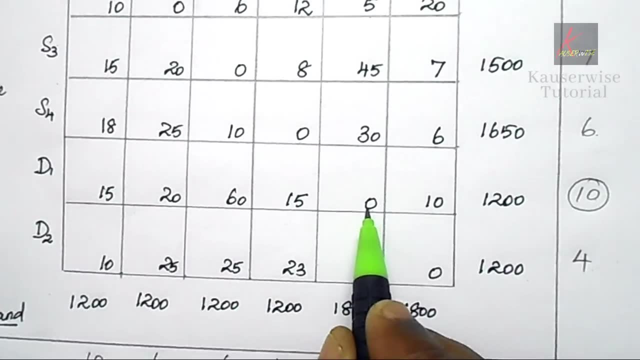 one. now i am going to select this particular row. in this particular row, i have to select the least value. so which one is least value? zero is the least value, so i am going to assign this particular cell by comparing demand and supply. demand for this particular cell is zero, so i am going to 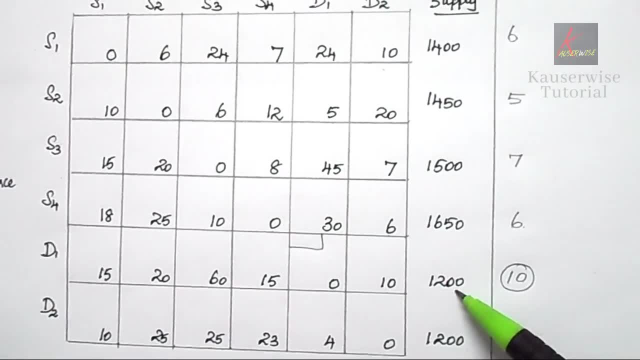 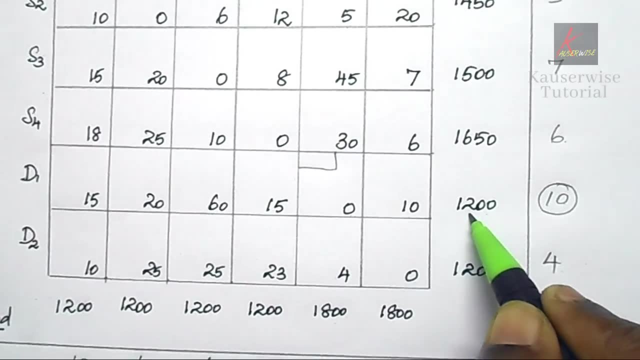 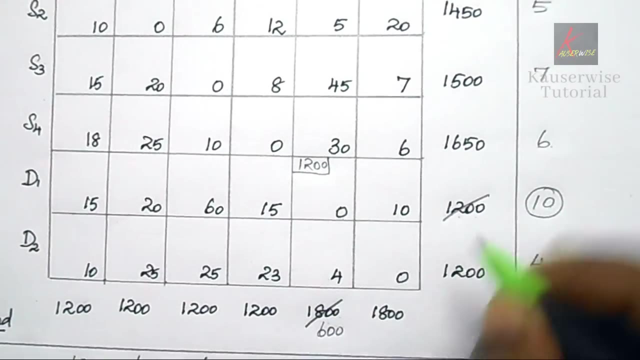 select. this particular cell is thousand eight hundred and supply is thousand two hundred. now compare the two values and assign the minimum value, so which one is minimum. thousand two hundred is a minimum value. so enter thousand two hundred here, and the balance is six hundred, here zero, because 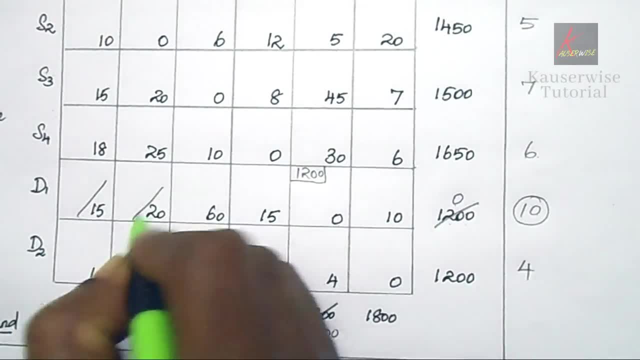 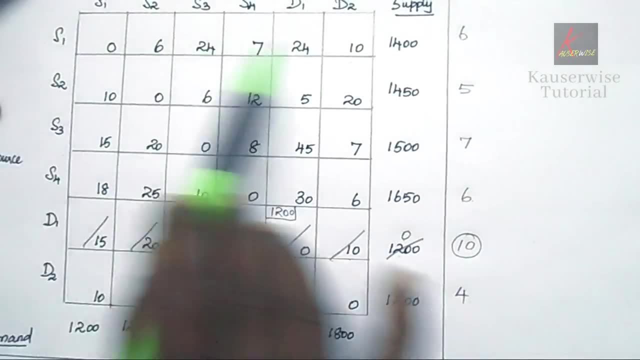 of zero, this particular row will get cancelled. so strike out. see again. we need to find the row difference and column difference for all other columns. so we are going to find the row difference- unallocated cell and we have to repeat the same procedure until we allocate all the demand and 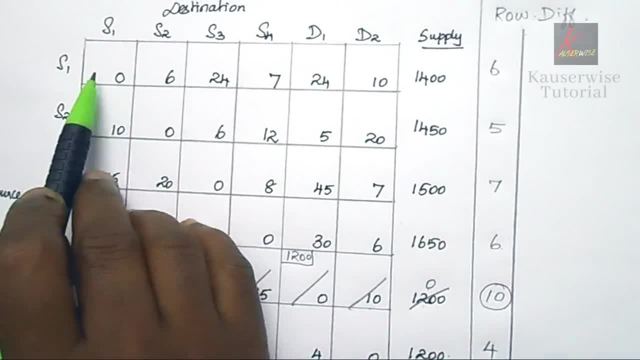 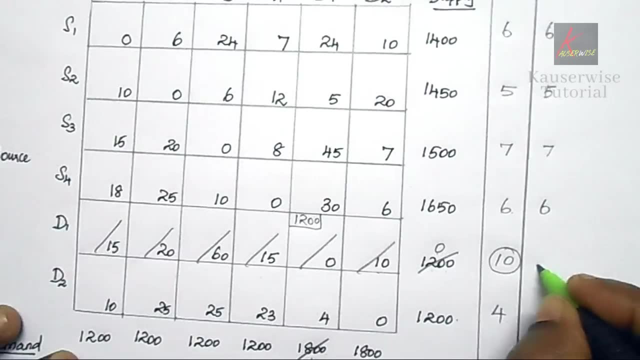 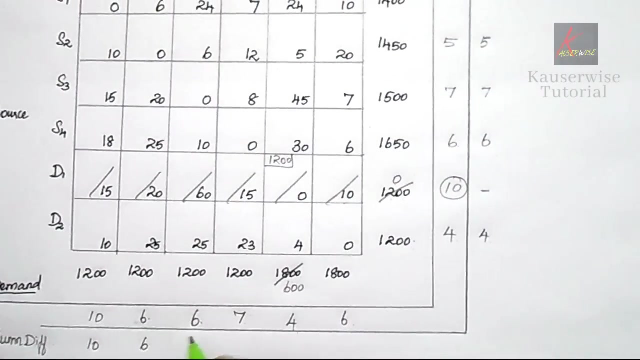 supply. again, we need to find out the row difference and column difference for the first row six. second row five. third row seven. fourth row six. here dash, next row four. in the same way, column difference for the first column ten. next is six, six, seven, one, six. now, after find out the row difference, 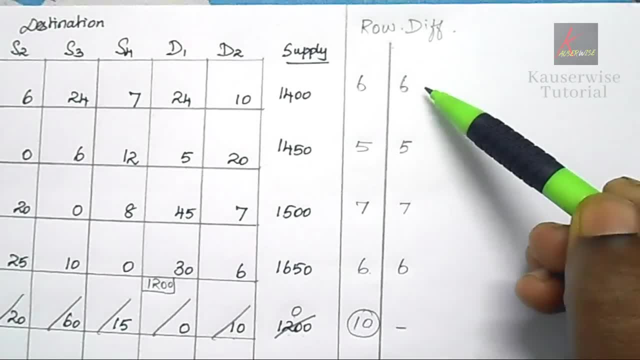 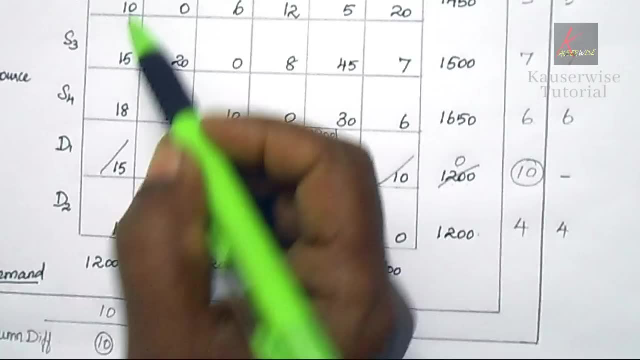 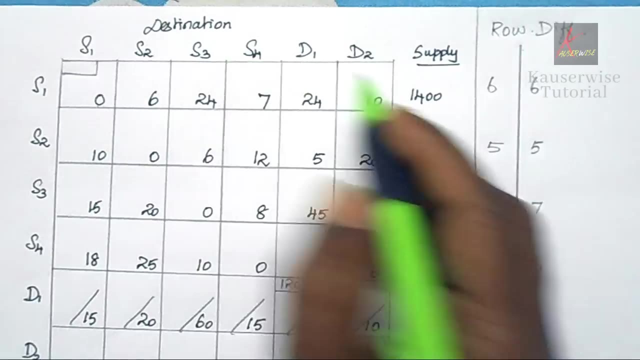 column difference. now we have to select the maximum difference. so which one is maximum value? yeah, ten is the maximum value. so select this particular column and select the least value in this particular column. so zero is the least value. so now compare the demand and supply. supply thousand. 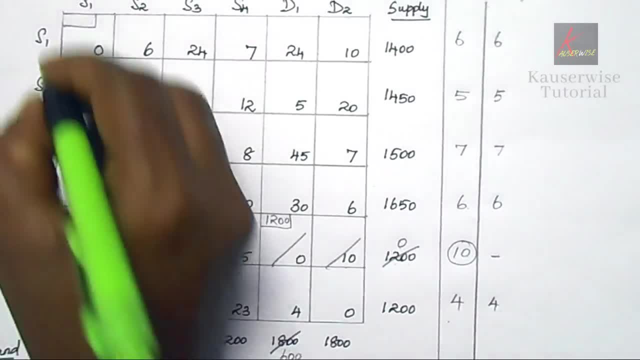 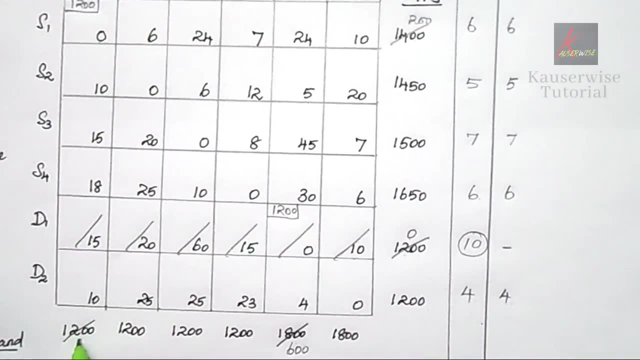 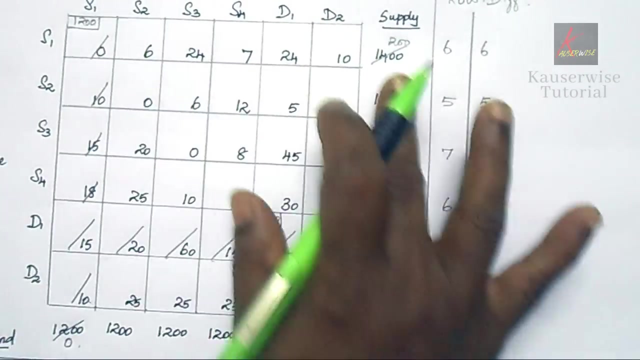 four hundred and demand thousand two hundred. so least value is thousand two hundred. allocate thousand two hundred, balance two hundred, here zero. so this particular column will get cancelled. see again, we need to find the row difference and column difference for all other unallocated cell and we have to repeat the same procedure. 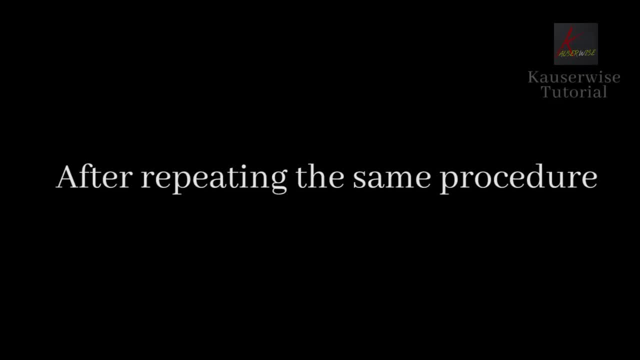 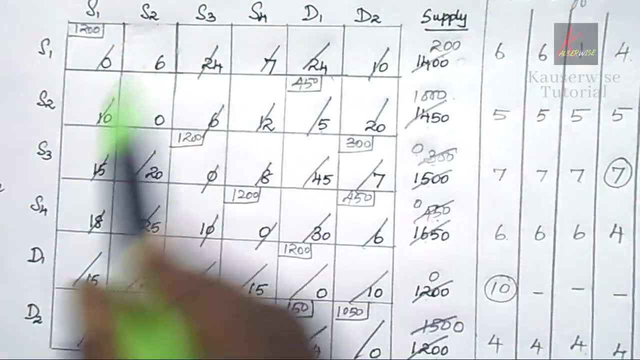 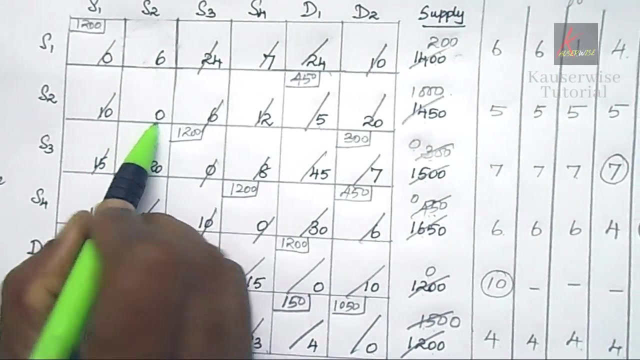 until we allocate all the demand and supply. see the matrix. now we have only two values. among these two values, which one is least? zero is the least. again, you need not find out any column difference and row difference. simply you can select one least value. so zero is the least. 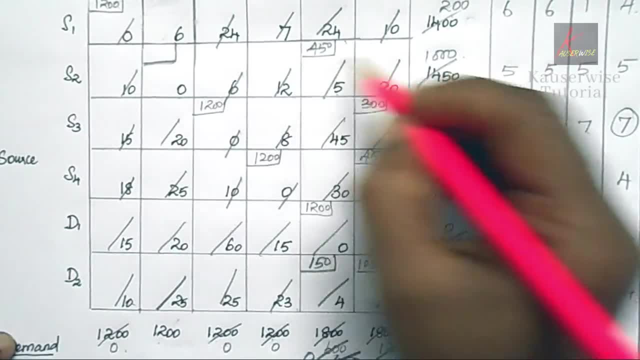 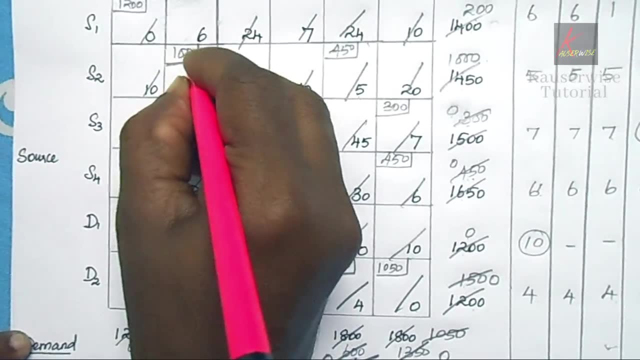 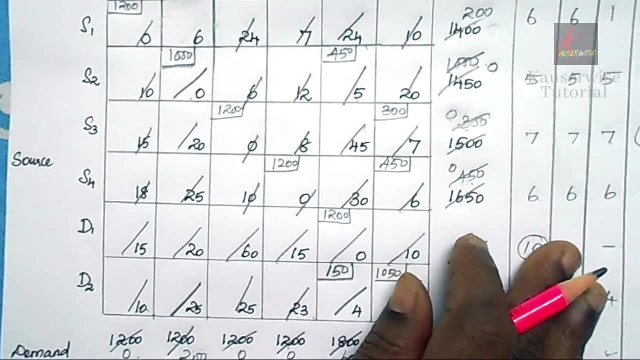 value. select this particular cell and compare the demand and supply: supply 1000 and demand 1200. so 1000 is the least value. assign 1000, 0, here 200, so this particular row will get cancelled. finally, we have only one cell in the last cell: demand and supply. both will be equal, just check. 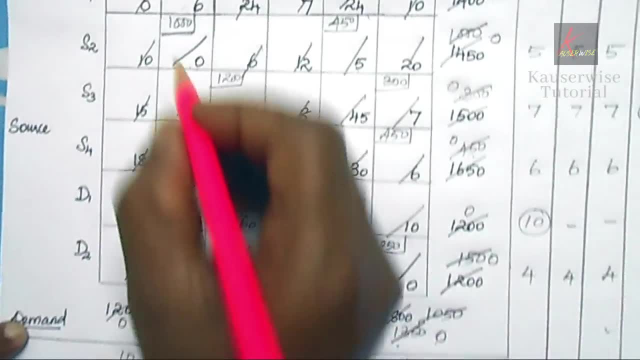 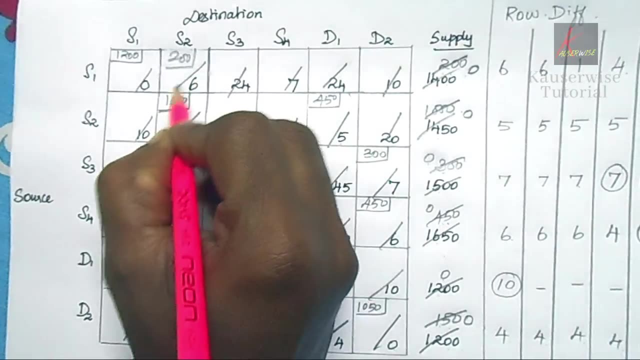 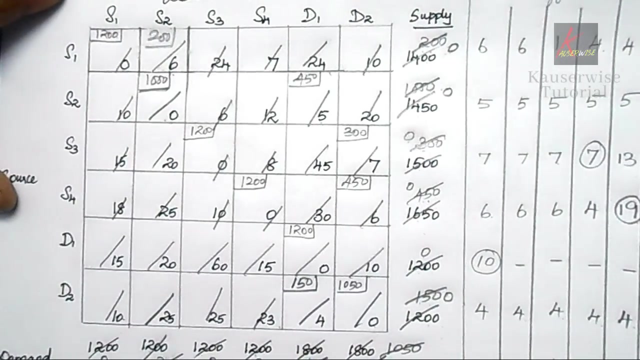 supply 200, demand also 200. so allocate 200 and put 0 here, also 0. this cell also will get cancelled. now just check whether we have allocated all the demand and supply. now we have allocated all the demand and supply. the entire cell got cancelled. now find out the total transportation cost. now i'm going to 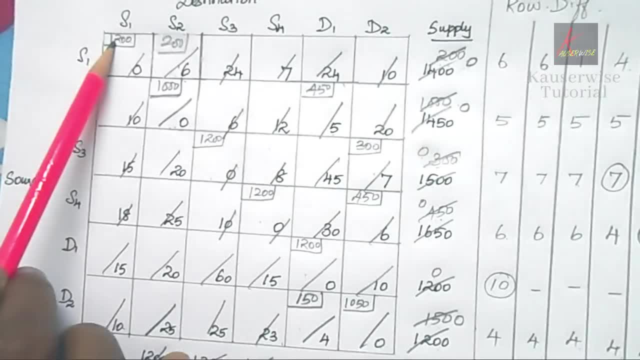 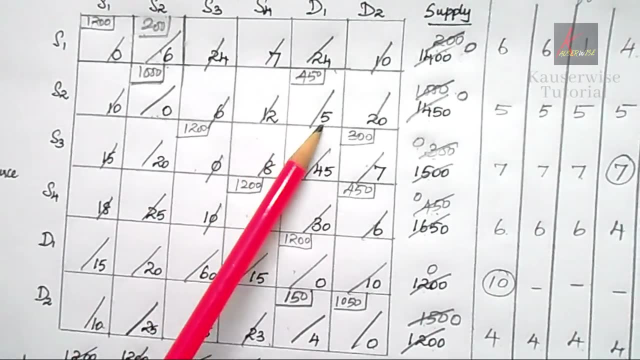 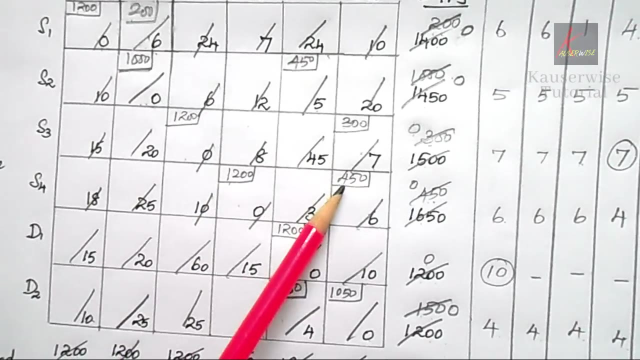 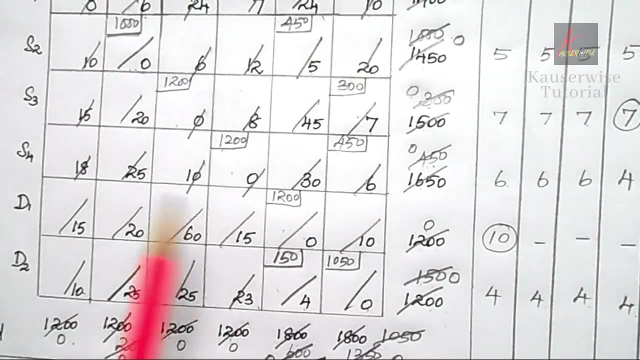 construct the new table with the allocated cells only: 1200 0, 206. 1000 0, 455. 1200 0, 307. 1200 0, 456, 1200 0, 150, 4 1050 0. these are the allocated cells. see when you. 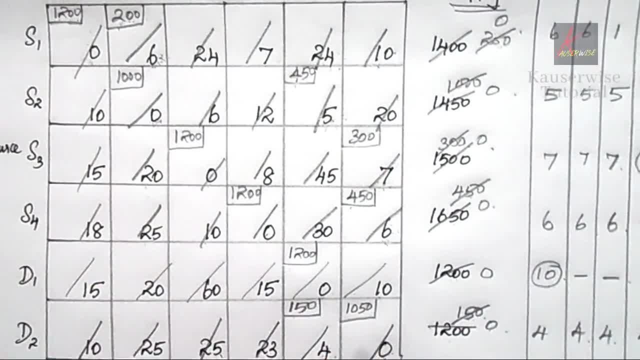 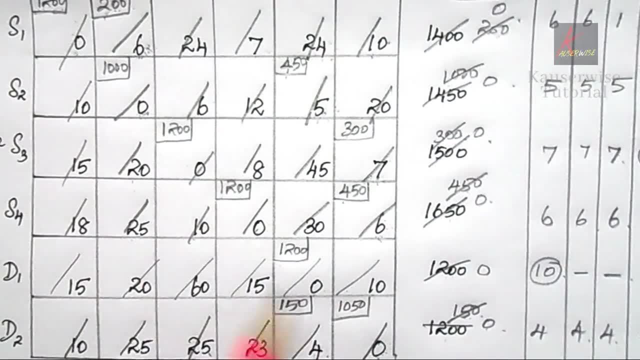 calculate the transportation cost. just ignore the zero values. anyway you're going to get zero only when you multiply any value with zero, you'll get zero only. just ignore all the zero and 50 and 50, 207 values. now i am going to find out the total transportation cost. just ignore the diagonal. 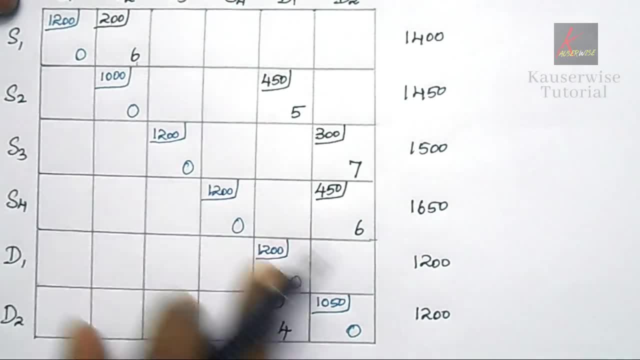 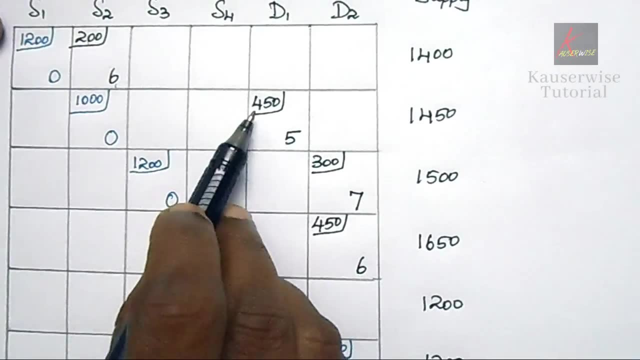 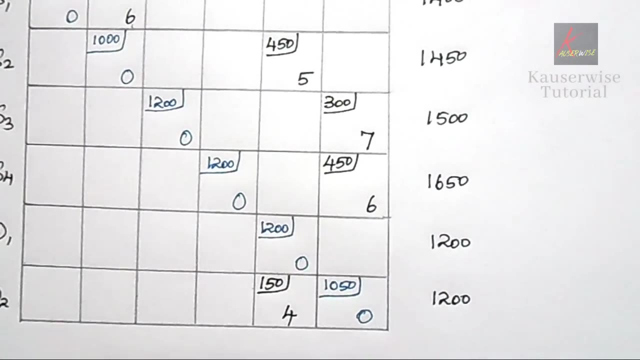 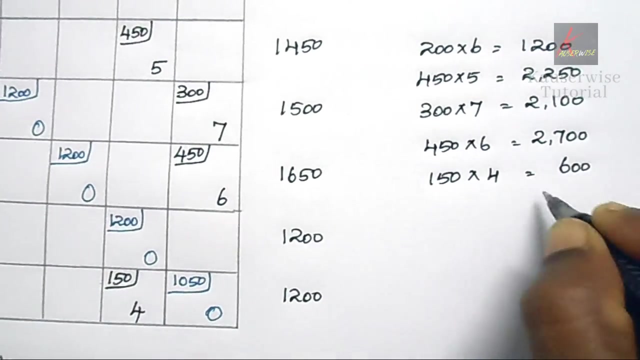 cell, because here we have got zeros. okay, ignore the diagonal cell and then only consider all other allocated cells here: 200 into 6 plus 450 into 5 plus 300 into 7 plus 450 into 6 plus 150 into 4, you'll be getting total transportation cost. so total transportation cost is 8,850. so this is the 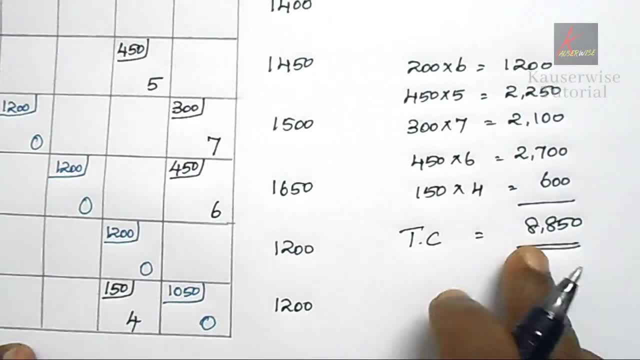 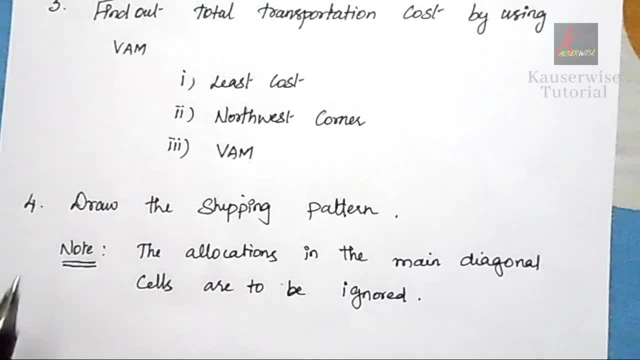 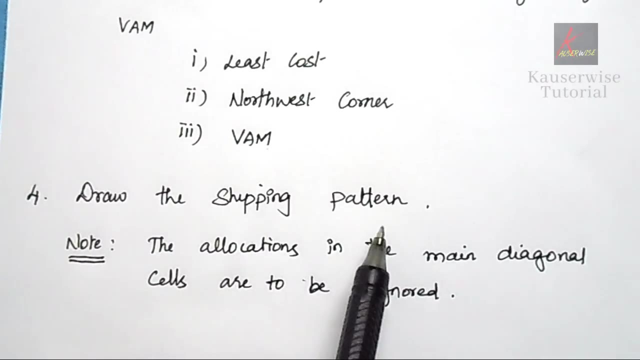 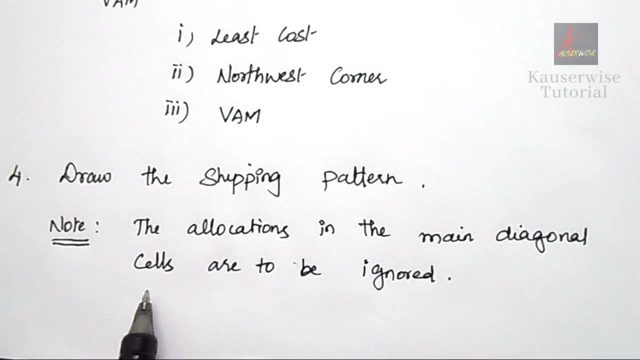 total transportation cost. okay, so 8,850. okay, after finding the total transportation cost, the last step is: look at the fourth step. after finding the total transportation cost, the last step is draw the shipping pattern. so here i'm going to draw the shipping pattern diagrammatically, by ignoring the diagonal cells. 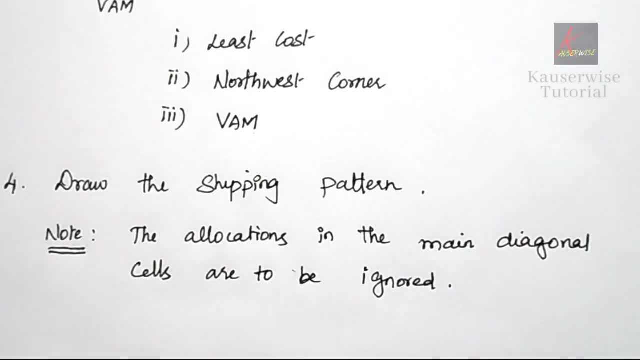 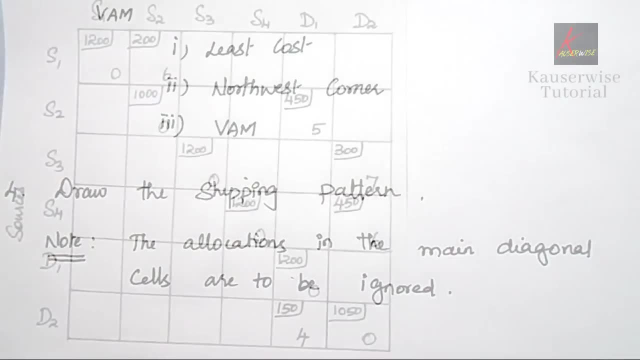 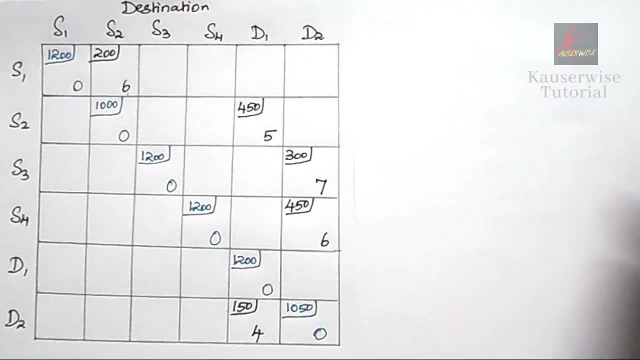 because the diagonal cells we have got zeros, no, so that just ignore the diagonal values and only take all other allocated cells and draw the shipping pattern diagrammatically. in this problem there are four sources and two destinations, so draw like this: so here sources, here destinations. when we draw the pattern, just ignore the main diagonal cells. 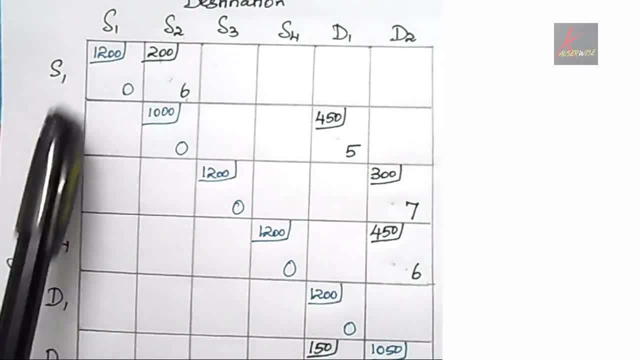 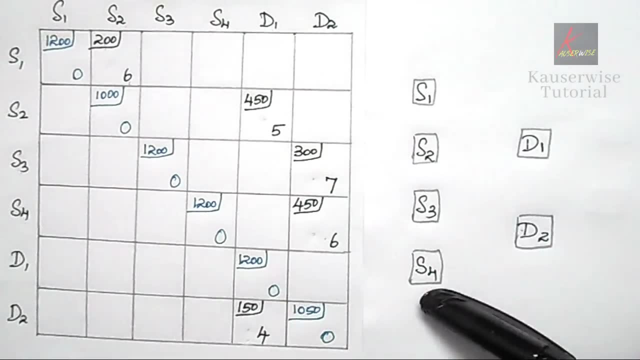 and we draw the shipping pattern and draw the shipping pattern. and draw the shipping pattern because it represent the same place: s1, s1, s2, s2, s3, s3. okay, so just ignore the zero values. first write the four sources and two destinations like this: look at the table. okay, in the first row. 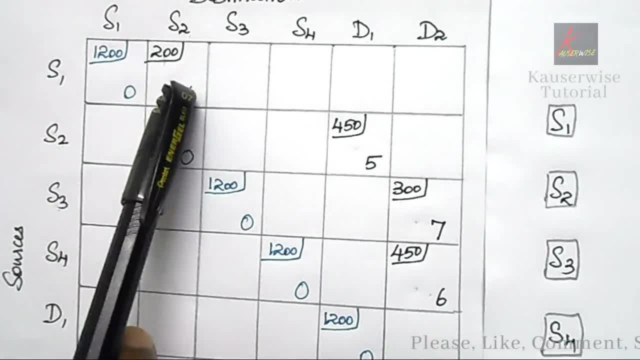 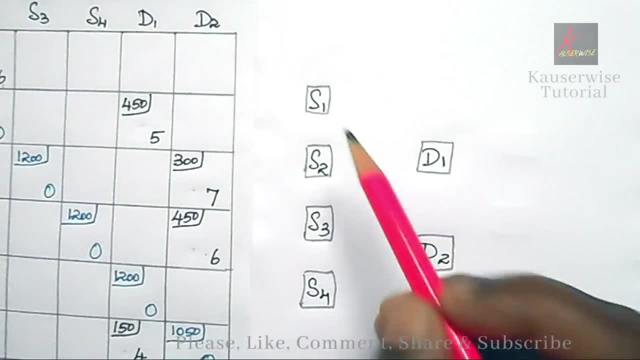 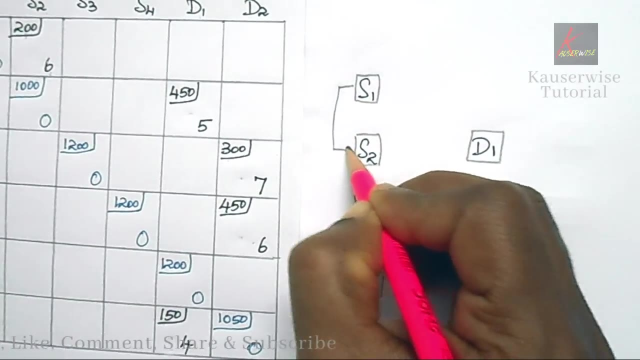 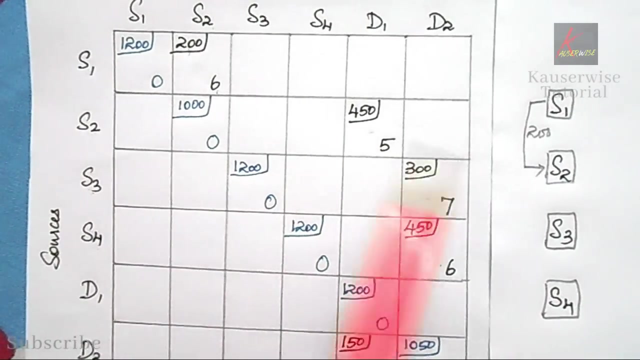 the allocated cell is located in s1 to s2. okay, so allocated value is 200. look at the pattern first: shipment starts from s1 to s2. the allocated value is 200. draw like this now see the table in second row: okay, the allocated cell is located in s2 to d1. 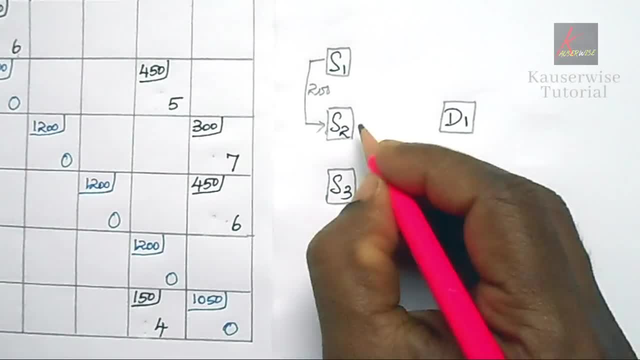 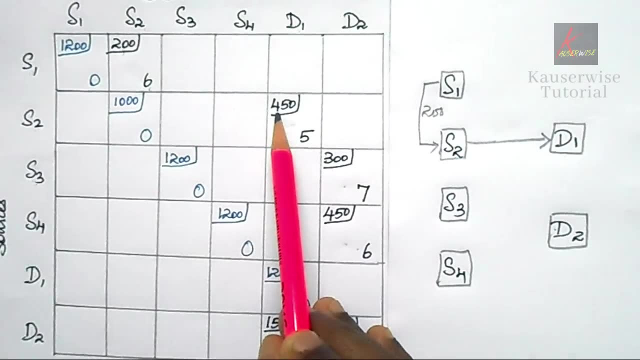 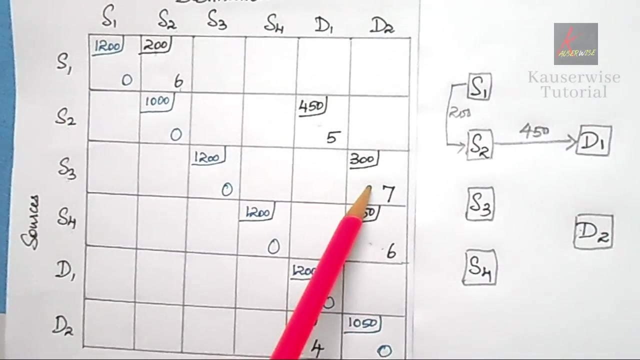 okay, from s2 to d1. it moves like this. the shipment moves like this: from s2 to d1. now see, the allocated cell is located in s1 to s2. okay, the allocated cell is located in s2 to d1, value 450.. So write 450 here. Look at the table in the third row, this is the allocated cell. it. 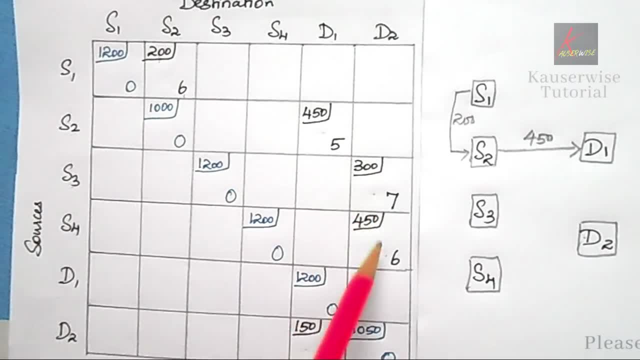 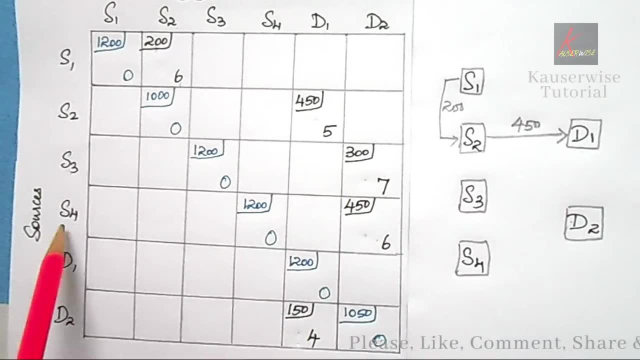 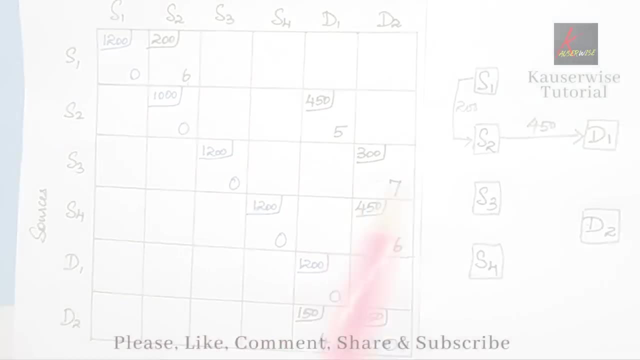 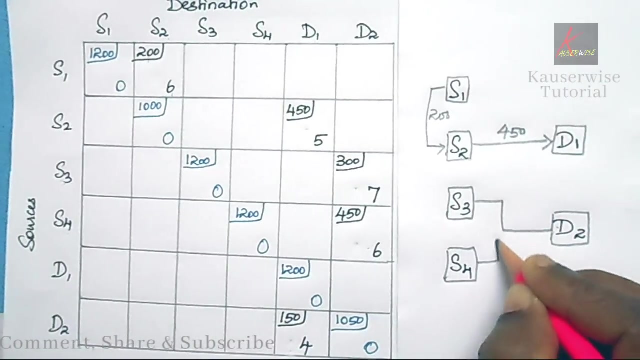 represent S3 to D2.. Again, we have one more allocation in D2, that is S4 to D2. So here S3 as well as S4, moving to same destination. Here the allocated value is 300, here 450.. Now draw the pattern like this: from S3 to D2 and from S4 to D2.. So both the sources reaches to. 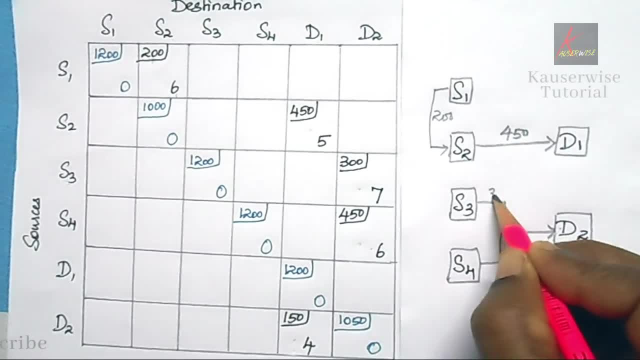 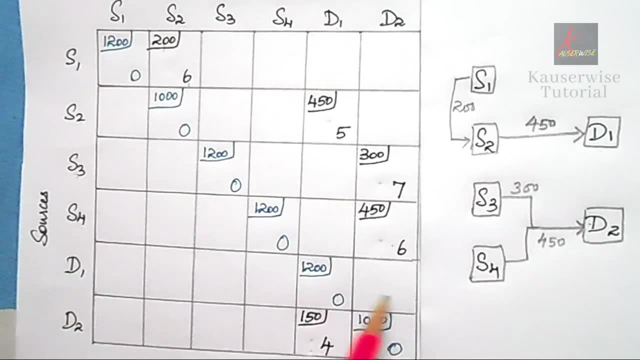 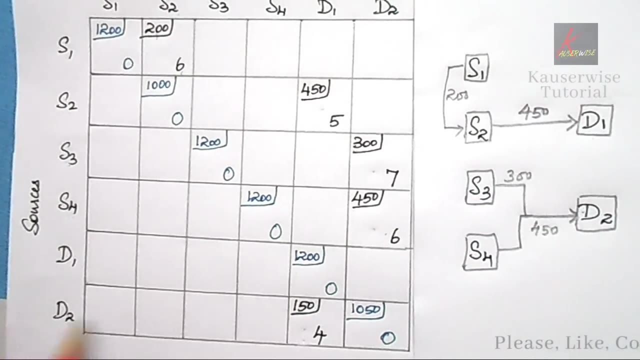 destination 2.. Okay, for here 300 is the allocated value, here 450 is the allocated value. Look at the table. in the fifth row there is no allocated value. See the last one. yes, here we have one allocated cell, that is. this particular cell represents D2 to D1..